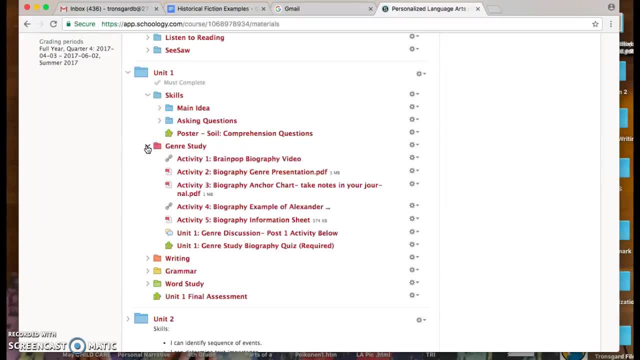 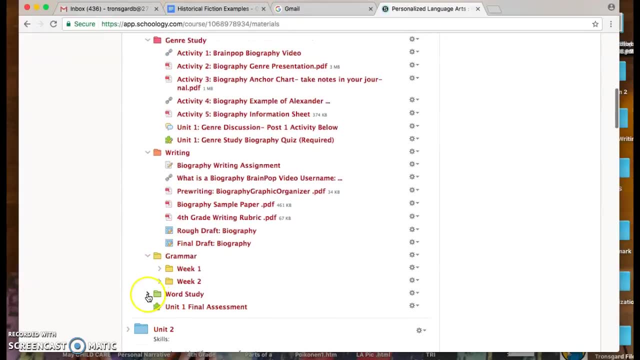 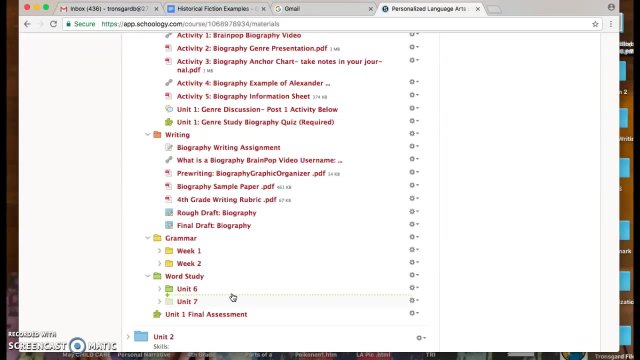 have to work on the genre study, writing, grammar and word study. So our units are two weeks long that we need to find a job that works for me. My name is켁 nin. We took them from three weeks down to two weeks. 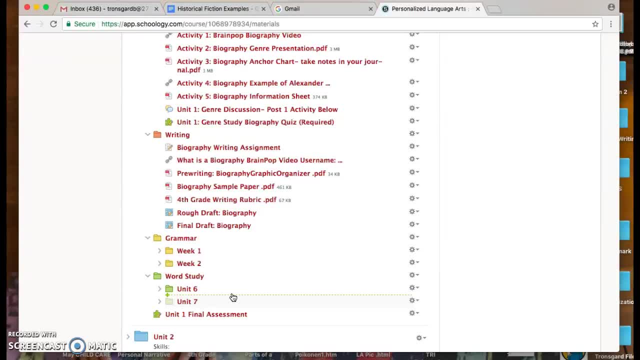 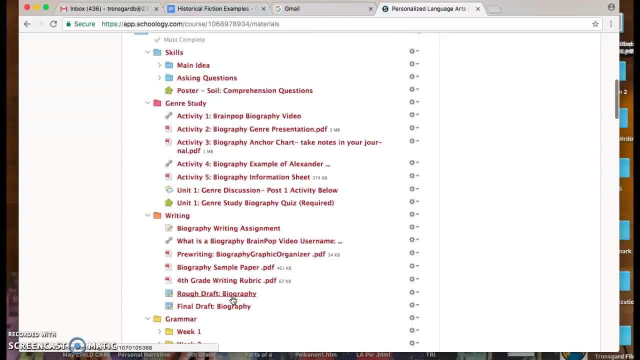 And so our word study. you will see, we will be starting this after the first 30 days of school, So we will be on unit six and seven. Each unit will have a post-test, a final assessment, to kind of see where our students are at. 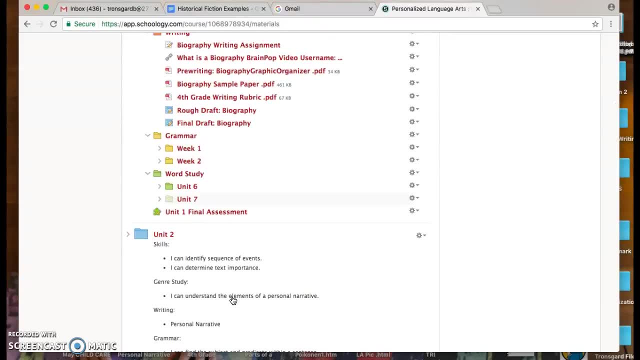 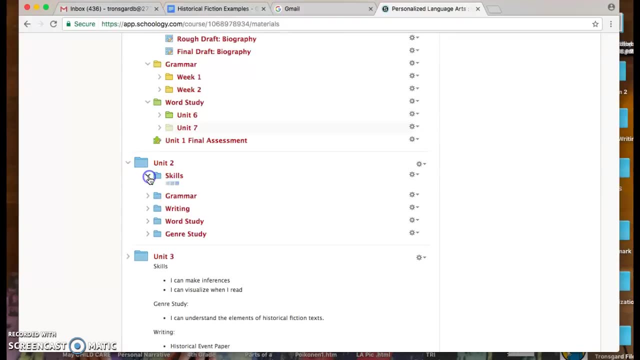 If they don't master this post-test, we will work with them to master that post-test before we let them move on to unit two. This is unit two and this is what I have been working on, And so, as students kind of come into the course, they'll see their skills are what we'll be working on in reading groups. 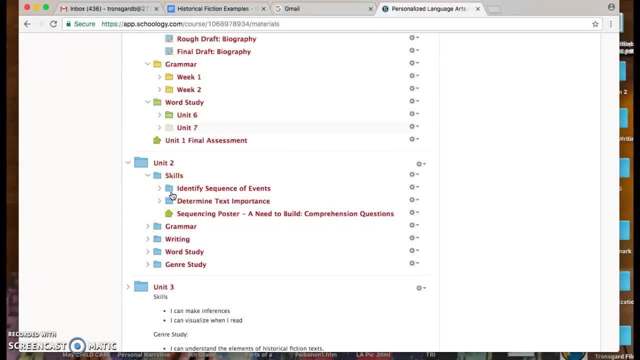 So identify sequence of events and determine text. importance are the skills in unit two, weeks one and two. In order to advance out of those skills, students will need to master the sequencing poster, a need to build comprehension questions. So that will give us an idea of what our students are struggling with. 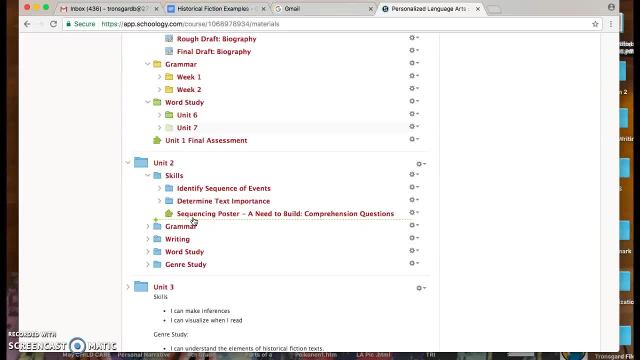 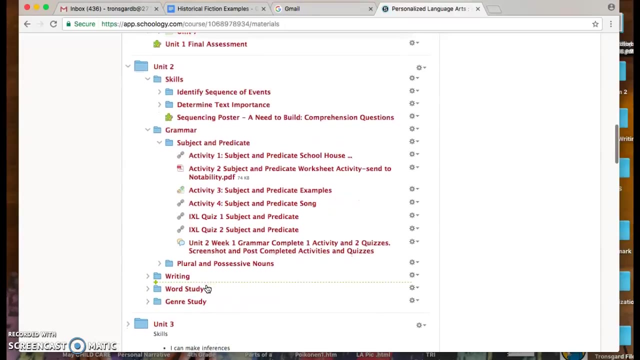 And how we can kind of help them advance on to that next skill. For grammar, you will find two different folders And within those folders you will see different activities that students can do. We'll be using IXL to quiz our students. 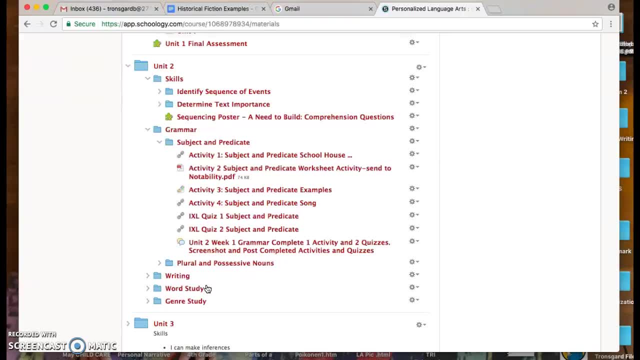 What's great about IXL is that it will kind of generate different quizzes to show us their mastery And then, once they master one of those quizzes, they will put in To our discussion their activity that they did and their two quizzes. Same goes for plural nouns. 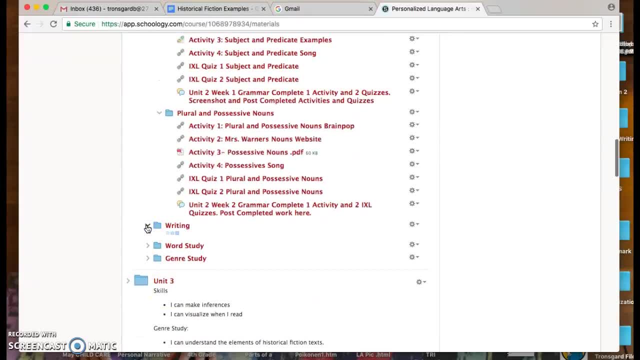 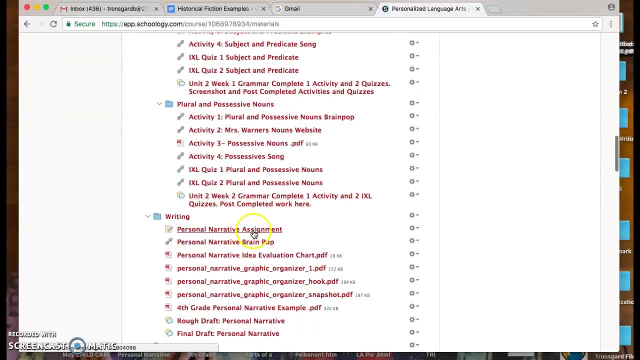 And then as we go into writing, each, every unit will have a writing prompt. So we will take the time to kind of explain that writing prompt but also give students the opportunity to kind of dive in a little more. Maybe they missed the lesson for that day.